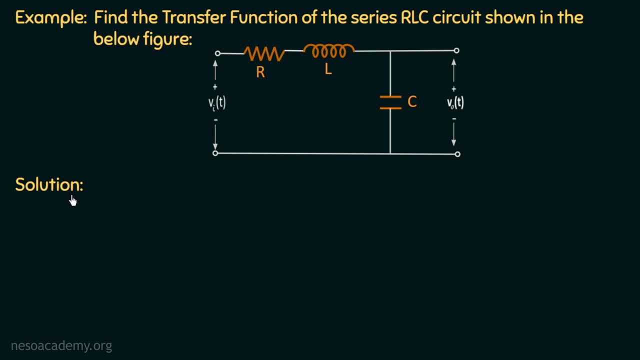 to calculate the overall transfer function of an electrical network, firstly we have to convert that network into its S domain. So if we convert this network into its equivalent Laplace domain, then the network will look like this: The input voltage is Vi, the 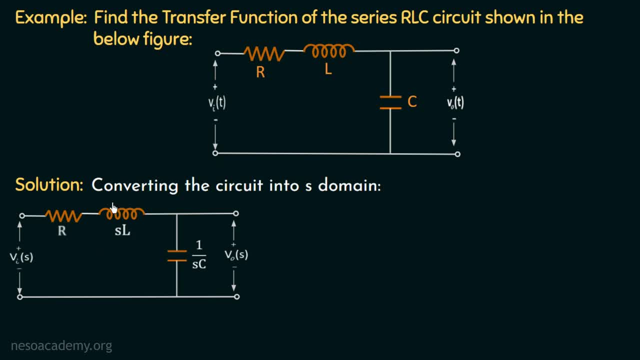 impedance of resistor is R, the impedance of inductor is Sl and the input voltage is V and the impedance of capacitor is 1 over Sc. The output voltage which is measured across the capacitor is V And we need to calculate the overall transfer function. 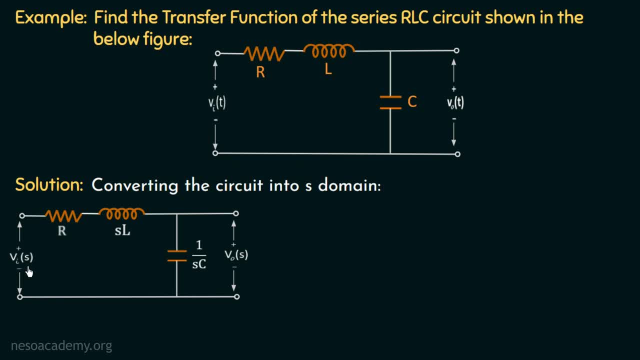 which is the ratio V over Vis In this circuit. we know that these three elements are present in series and we can calculate this output voltage by using the voltage divider rule. So, firstly, we will calculate this output voltage across this capacitor by using the voltage divider rule. 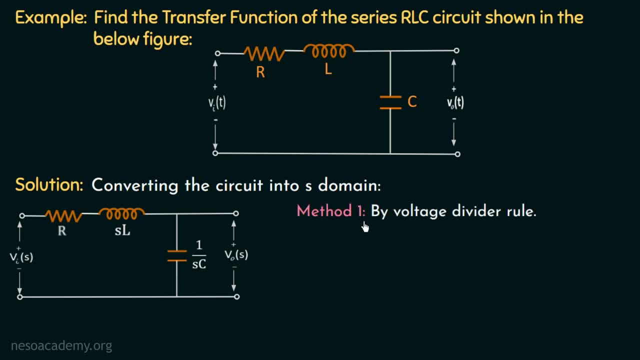 So this is our method number one, in which we will apply the voltage divider rule. So we have V out of S, which is the output voltage, equal to 1 over Sc, which is the impedance of this capacitor over R plus Sl, plus 1 over Sc, which is the total impedance. 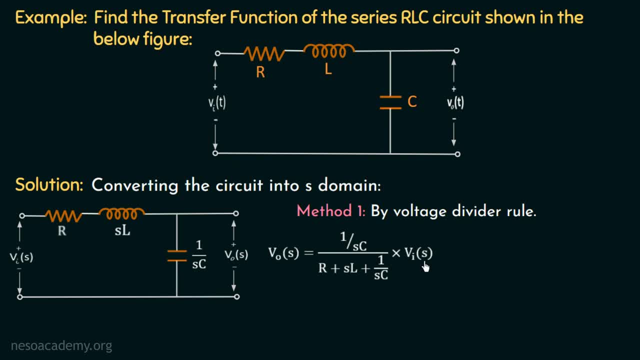 of this complete circuit multiplied with Vi, which is the input voltage. Let us check this one more time. We have three elements present in this circuit. the first one is the resistor having impedance R, the second one is the inductor having impedance Sl and the third one is the capacitor having impedance 1 over. 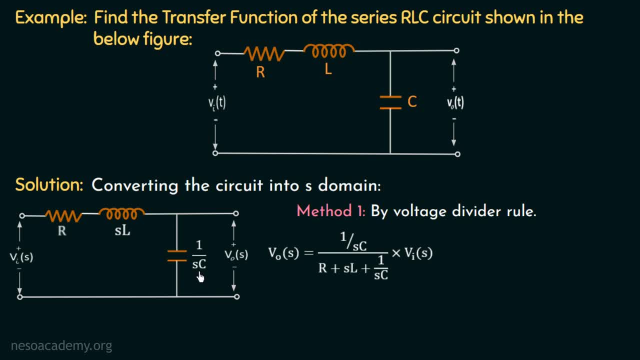 Sc. If we want to calculate the total impedance of this circuit, then it will be R plus Sl plus 1 over Sc, since these three elements are present in series. Now, if we want to calculate the output voltage measured across this capacitor, then it will be equal to Vi. 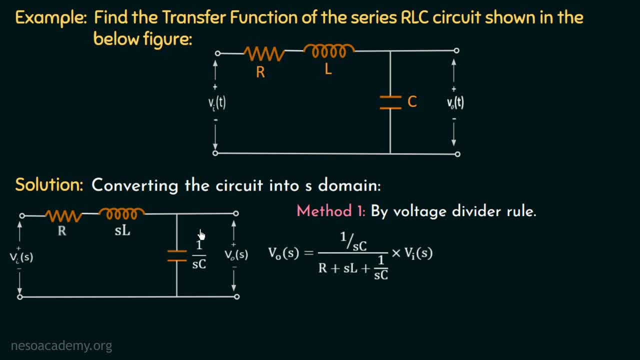 equal to 1 over Sc, which is the impedance of this capacitor over the total impedance multiplied with the input voltage, which is Vi. Now if we take the LCM in the denominator, we will have V equal to 1 over Sc, over R plus S squared multiplied. 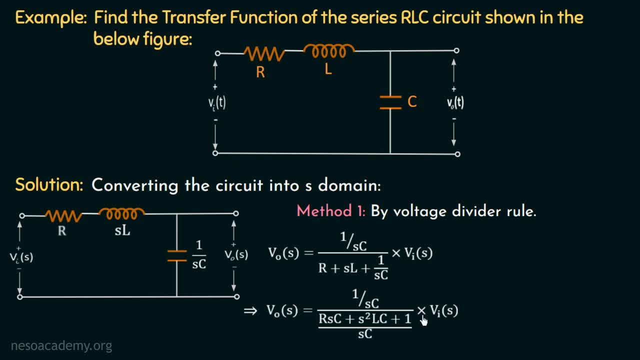 with LC plus 1 over Sc, which is multiplied with Vi. Now we can see that this term in the denominator and this 1 over SC will get cancelled and we will have the overall transfer function Vout S over Vis equal to 1 over S squared multiplied with LC plus RSC plus 1.. 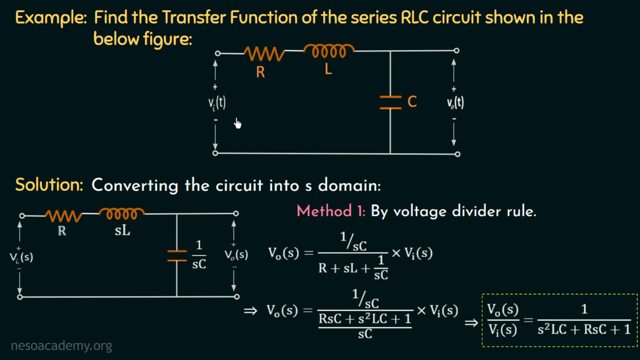 And this is the overall transfer function of a series RLC circuit, and we have calculated this by the use of voltage divider rule. So in this way we are done with the calculation of transfer function of this series RLC circuit by using the voltage divider rule. We will now move on to the 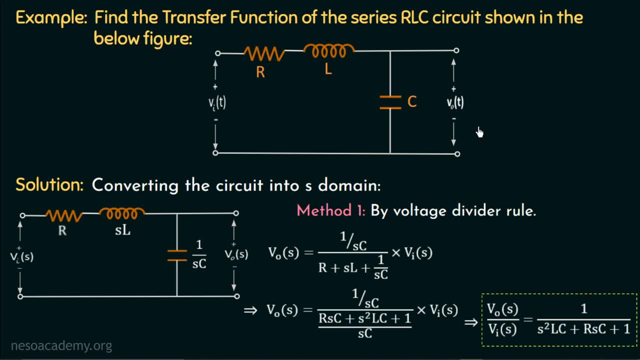 method number 2, in which we will model this electrical network, That is, we will convert this series RLC circuit into a signal flow graph and then we will calculate the overall transfer function by using the Mason's gain rule. Moving on to method number 2,, which is the 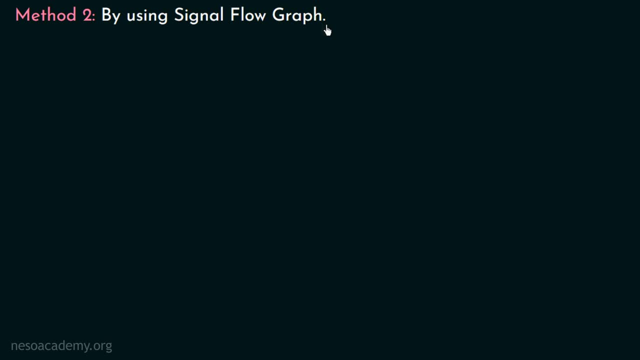 calculation of transfer function by using the signal flow graph. So let us consider the given electrical network 1 and 2.. One more time. we have a series RLC circuit in which the impedance of resistance is R, the impedance of inductor is SL and the impedance of capacitor is 1 over SC. 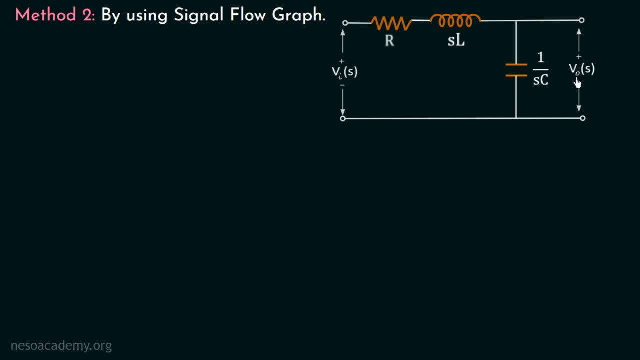 The input voltage is Vi of S and the output voltage which is measured across the capacitor is V out of S. And now we will try to convert this complete electrical network into its equivalent signal flow graph, And for that sake we have to calculate the branch current. 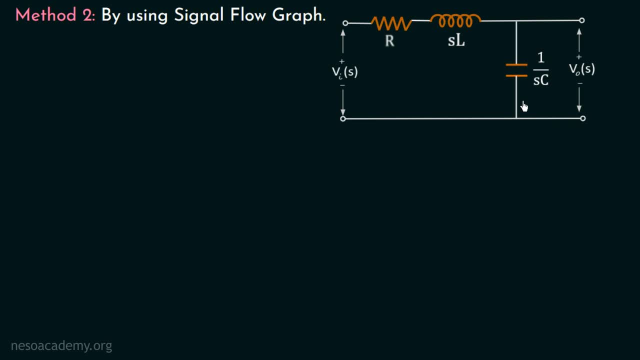 equation and the node voltage equation. So let us assume the current in this loop equal to Is, as we know that the current in these three elements will be the same. Moreover, the output voltage is V out S, which is measured across this capacitor and hence the voltage. 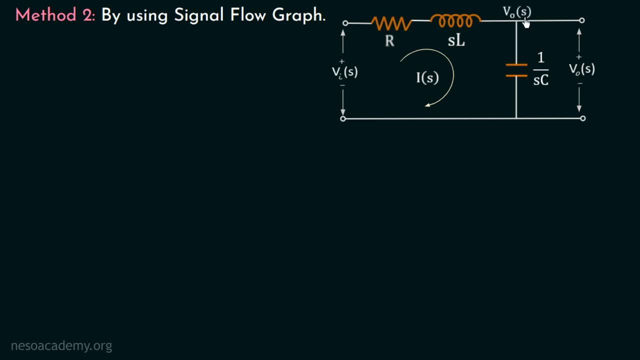 at this particular node will be V out of S. Now we have to write the equations for this branch current equation. So firstly, let us try to write the equation for this branch current Is. We know that this current Is is same in all the three elements, as the three elements are present in series. 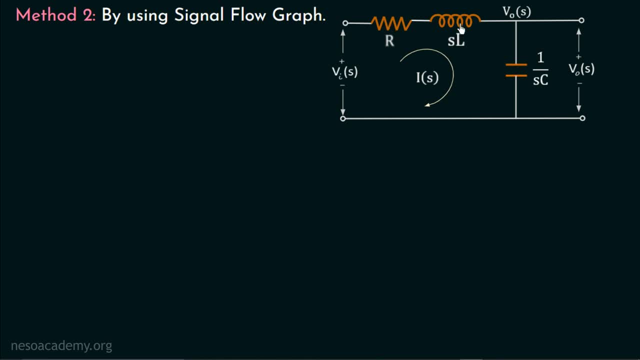 And that's why we can say that the current in this resistor and this inductor is Is. Now, in order to find out the current Is, we can apply the Ohm's law in this branch. We know that the voltage at this resistor is V out of S and the output voltage is V out. 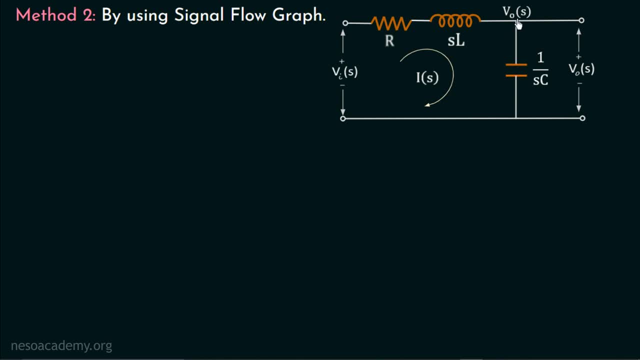 of S And the amount of OL at this terminal is just like the number of props used in our HypeStorm Materials. Now we definitely cannot2, not set. if it is going to be is equal to Is equal to Ohm's law. So what happen is that the voltage at this terminal is VI of S and the voltage at this inate is V out of S And the total impedance will be R plus SL. So we can write: Is equal to V fallen minus Vs And the total impedance of this branch will be R plus SL. So we can write, or we can write. I s equal to VI of s minus Vout of s over Rsl. Since this resistor and the inductor are present in series, we can add the impedances of these 2 elements and hence we have Is equal to VI of S minus V0 of s. There is value of this, value of R, as YouTube will say: individuals. 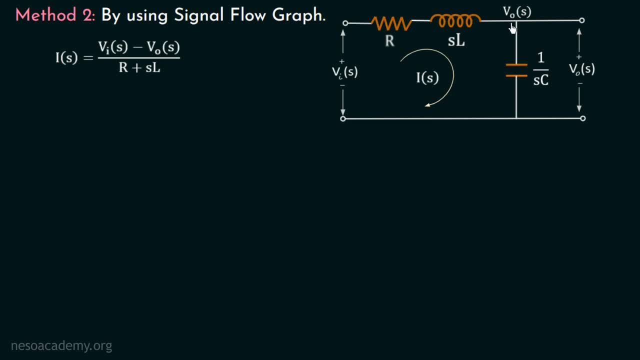 minus V0 of s, which is the voltage difference between these two nodes over the total impedance R plus SL. Now if we split this term, we have Is equal to Vi of s over R plus SL, minus V out of s over R plus SL, and this is the branch current equation. Now we will move on to the 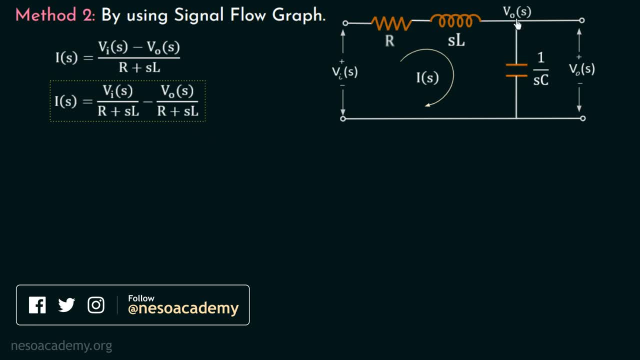 calculation of this node: voltage V out of s is the voltage drop across this capacitor, and we know that the voltage drop across any element is the current passing though that element multiplied with the impedance of that element. So we will have V out of s equal. 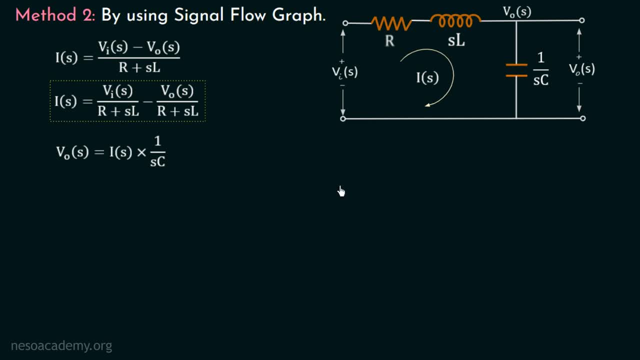 to Is multiplied with 1 over Sc- See the current passing through this capacitor- is Is, as all the three elements are present in series and the impedance of this capacitor is 1 over SC. So IS multiplied with 1 over SC will be the voltage drop across this capacitor. 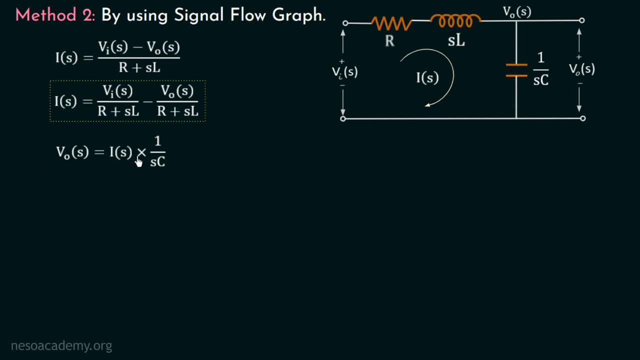 and hence V out of S will be equal to IS multiplied with 1 over SC. And this is our second equation, which is the node voltage equation. Now, as we have these two linear equations, we can now draw the signal flow graph of this electrical network. And we know that a signal flow graph 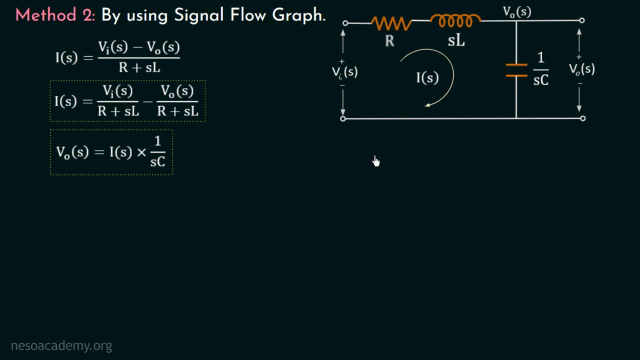 consists of nodes and branches And the nodes represent the variables, And in an electrical network the variables are the voltages and the currents. And in this network we have 2 voltages, VI of S, V out of S and 1 current, which is I of S. So in the signal flow graph, 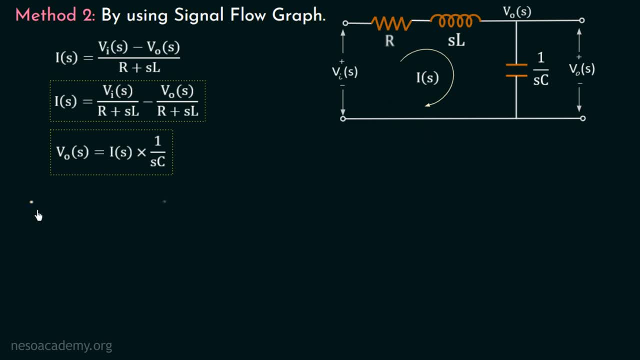 representation of this network. we will have 3 different nodes. The first node will be VI of S, which is the input voltage. This node will be V out of S, which is the output voltage, And this node will be I of S, which is the branch current. Now, if we observe this branch current equation, which 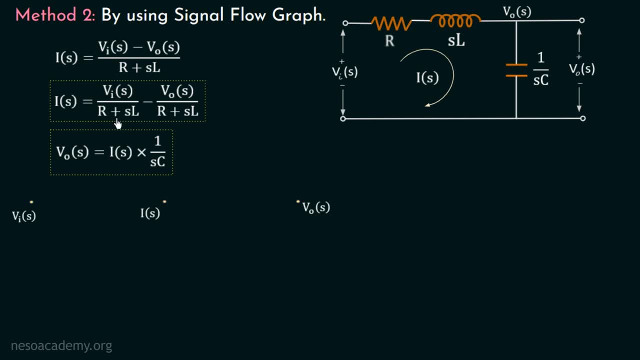 is IS equal to VIS over R plus SL, minus V out S over R plus SL. We can see that this equation relates this node IS with this node VIS and this node V out of S. We can see that this node IS is equal to VIS multiplied with IS over R plus SL, plus VIS multiplied with. 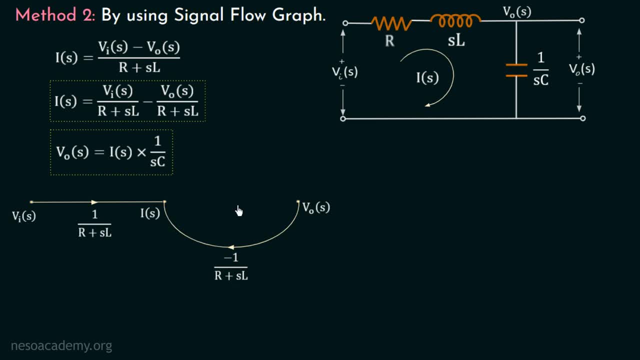 minus 1 over R plus SL. In this way, we have satisfied this first equation. We will now move on to the second equation, which is VIS equal to IS multiplied with 1 over SC. We can see that this equation relates this node IS and this node V out of S, And we can see: 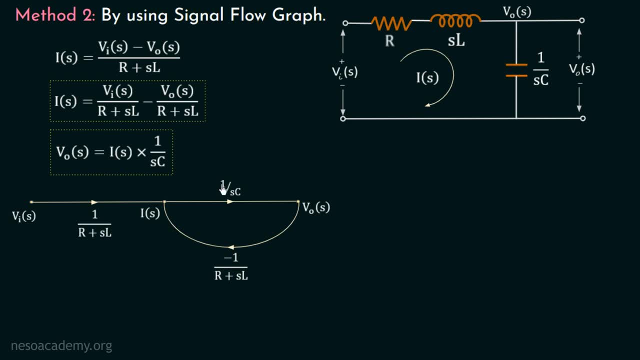 VIS is equal to I of R plus SC. So we can see that we can now move on to the next equation, which is VI out of S, which is I of S multiplied with 1 over R plus SL. We can see that this is equal to IS multiplied with 1 over SC, And this is the complete signal flow graph. 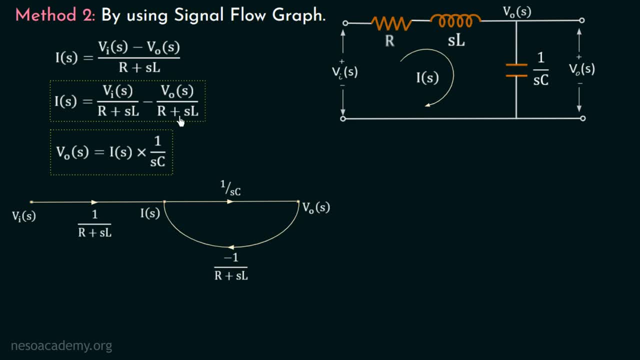 of this electrical network, And we have drawn this by the use of these two equations. Now, as we have the signal flow graph of this electrical network, we can now apply the Mason's gain rule in order to find out the overall transfer function. So, firstly, we have to 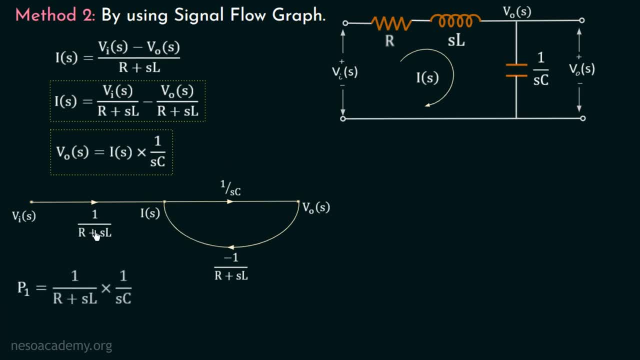 calculate the forward path gain, which is the product of these two branch gains, which is 1 over R plus SL multiplied with 1 over SC. Now we have to calculate the loop gain. There is only one loop present in the signal flow graph and the loop gain will be the product of. 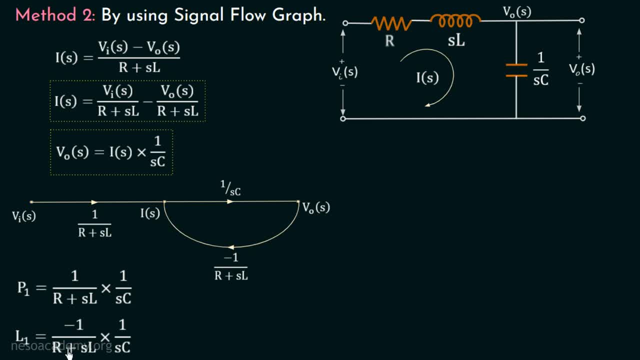 these two branches, It will be equal to minus 1 over R, plus SL, which is the branch gain of this branch, multiplied with 1 over SC, which is the branch gain of this branch. Now we will calculate the determinant of SFG, which is delta E. 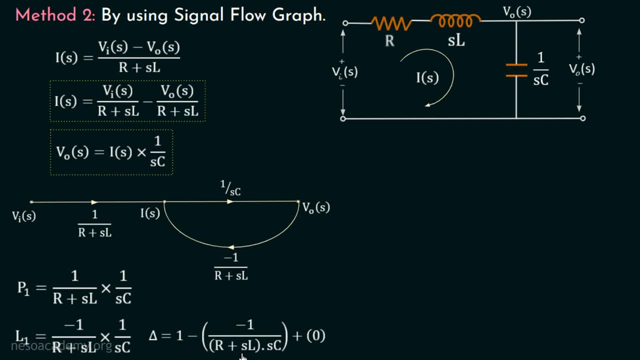 Delta E is equal to 1 minus of all the individual loop gains In this signal flow graph, we have only one loop having gain minus 1 over R plus SL multiplied with 1 over SC. So we will have delta equal to 1 minus of minus 1 over R plus SL multiplied with SC plus 0.. As we do not have any, 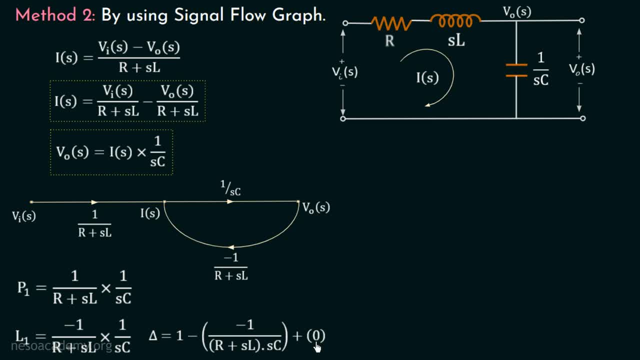 non-touching loops. in this signal flow graph, the gains of all the non-touching loops will be equal to 0.. Solving this, we will have the determinant equal to 1 plus 1 over R plus SL multiplied with SC. Now, lastly, we will calculate the associated path factor del 1, which is equal to 1,. 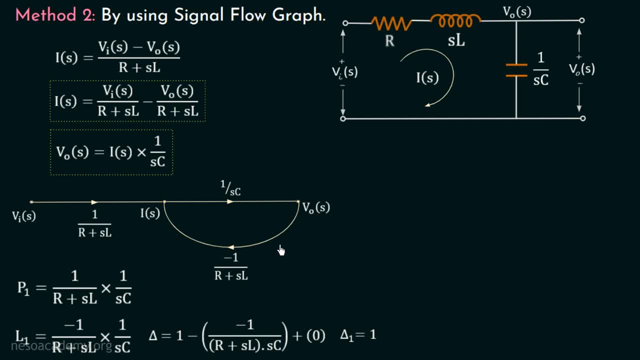 as we do not have any isolated loop in this signal flow graph, Now we will apply the Mason's gain formula in order to calculate the overall transfer function. We will have: V out S over V IS equal to P1 multiplied with del 1 over del. 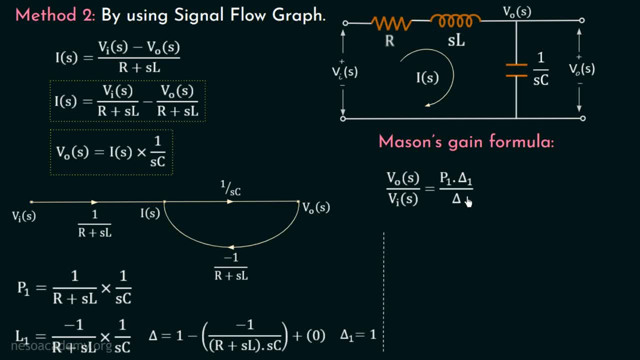 delta. And now, if we put all these values in this equation, we will have V out. S over V IS equal to 1 over R plus SL multiplied with SC. over 1 plus 1 over R plus SL multiplied with SC. The forward path gain P1 is 1 over R plus SL multiplied with SC. The value of associated 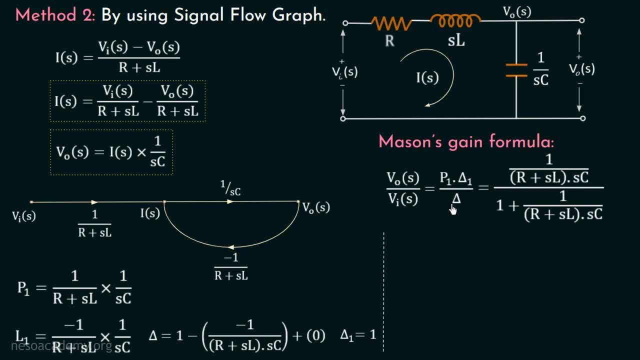 path factor is equal to 1 and the value of determinant of SFG is 1 plus 1 over R plus SL multiplied with SC. Now if we take the LCM in the denominator, we will have Vout S over Vis equal to 1 over R plus SL multiplied with SC over R plus SL.